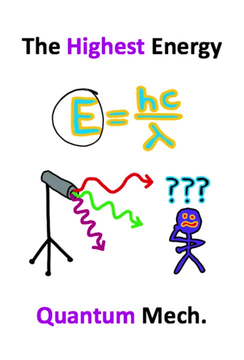 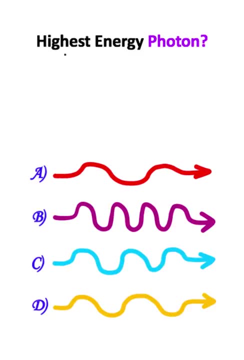 the wavelength shows up on bottom of this fraction. That means that the energy and the wavelength are inversely related to each other. So let's say I draw four different light waves on the screen and I ask you to find the light wave that has the highest energy.